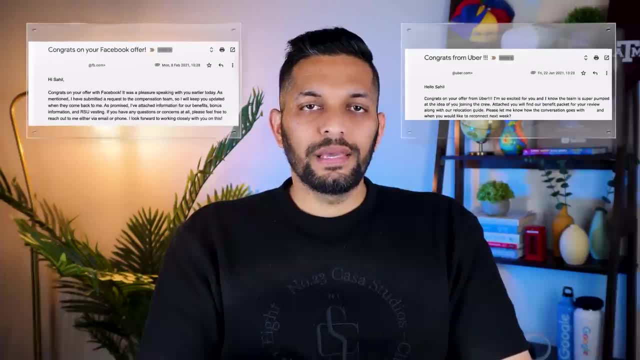 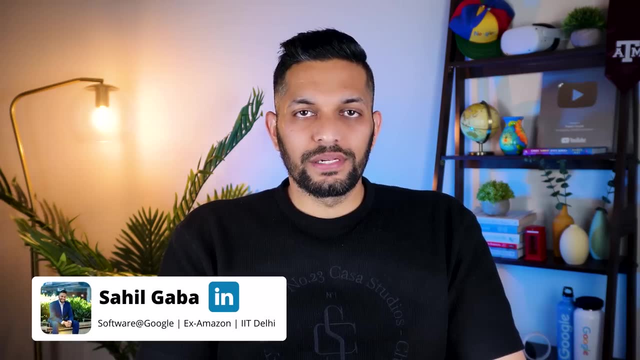 more than 500 problems on Leetcode, And along the way, I collected many amazing job offers. Today, I'm going to share everything that I've learned in the process. At the end of the video, I'll also answer a very important question, And that is: 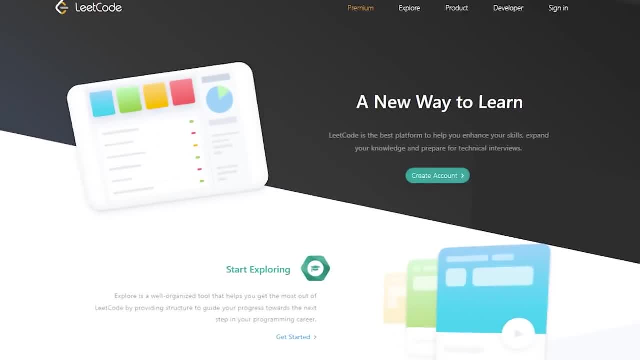 How do you solve problems in Leetcode? How do you solve problems in Leetcode? How do you solve problems in Leetcode? How to know if you're ready for interviews at big tech companies. Before you can even start on Leetcode, you need to have a good 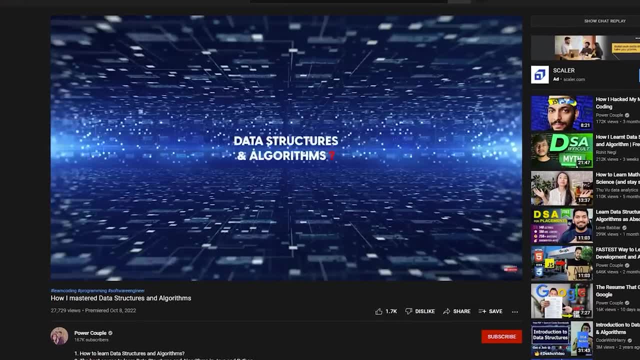 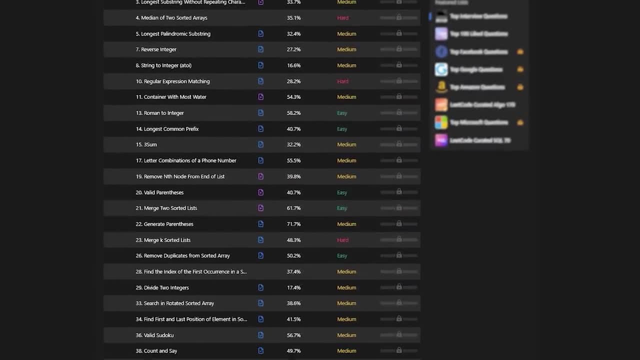 understanding of data structures and algorithms. I have already covered this topic in my last video, which I'll link at the end. Once I finished the basics of DSA, I went to the top interview questions on Leetcode. There are exactly 150 problems in there and all. 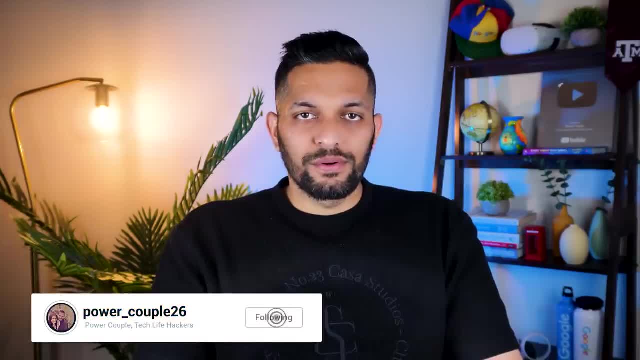 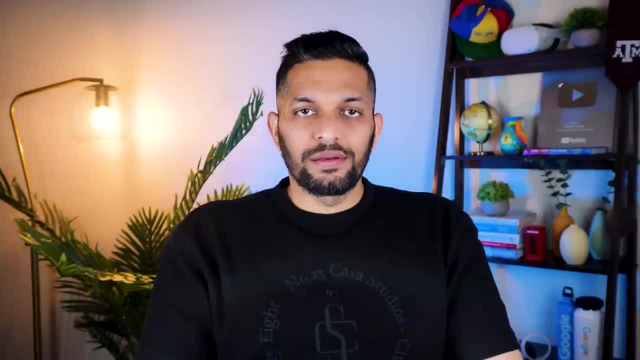 of them are very important. I recommend that if you're solving a problem which is outside these 150 problems, make sure it's your 151st problem. Now that you know where to start, let's discuss what's the right strategy to solve these problems. I'm sure that you already know that all the problems on Leetcode 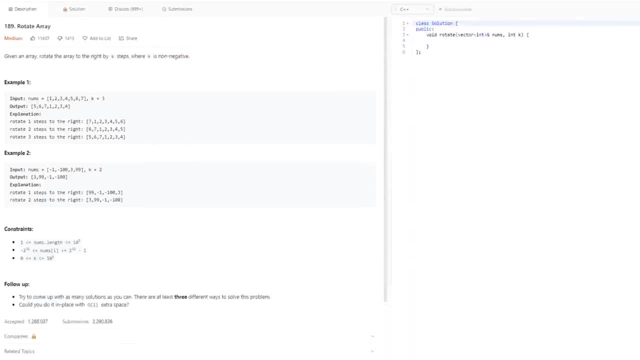 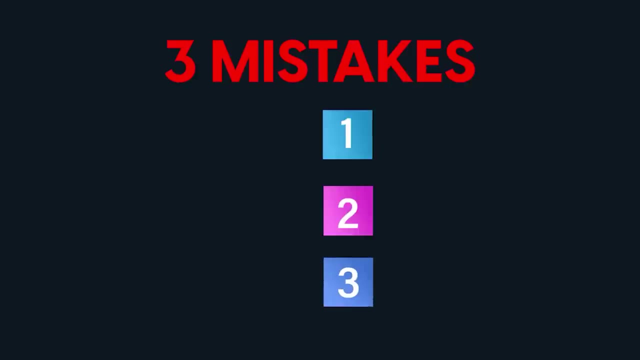 are tagged easy, medium or hard based on the difficulty level And if you look a little closer at the rotate array problem, which was my first problem on Leetcode, it's tagged as a medium difficulty problem. Starting my Leetcode journey with this problem was my. 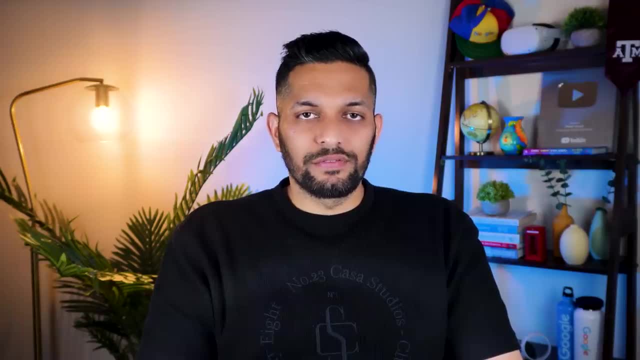 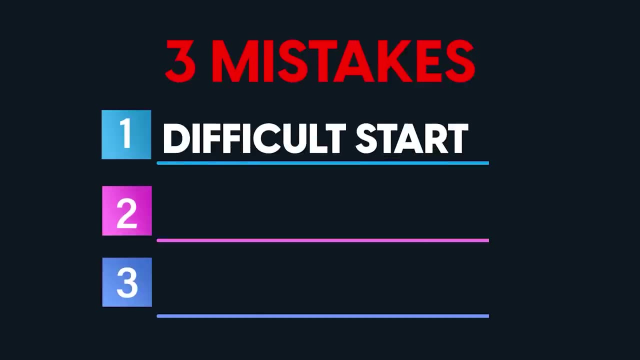 first big mistake. I made two other mistakes that I'll share later in this video. This problem was a mistake because if you're looking to stay motivated and actually improve your programming logic, you have to start with the easy problems, As you solve some easy. 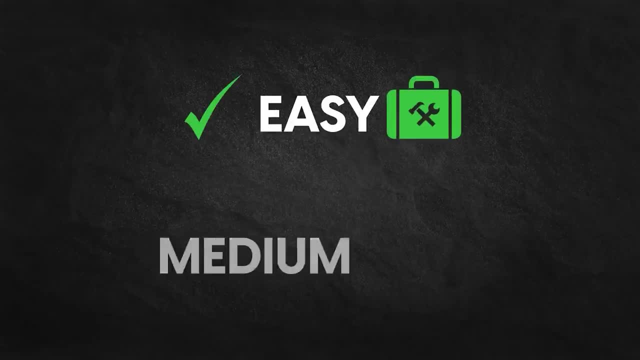 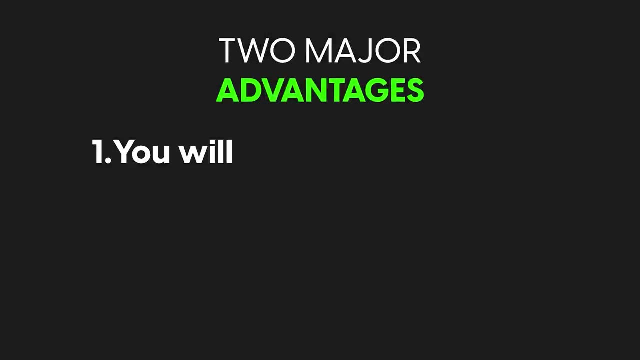 problems, you'll start collecting some tools to solve them. You'll start collecting some tools for your toolbox And when you reach the medium problems, you'll be able to use these tools to tackle them. This approach has two major advantages. One: you will not lose your confidence like I did. 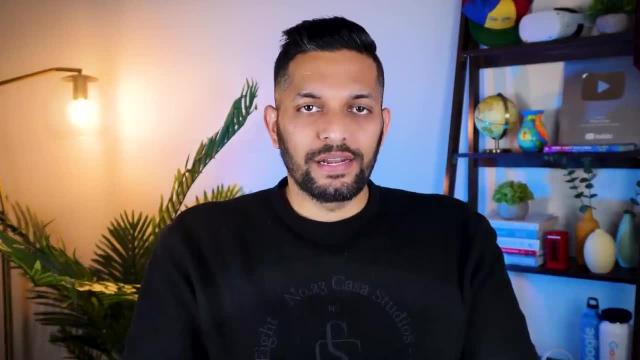 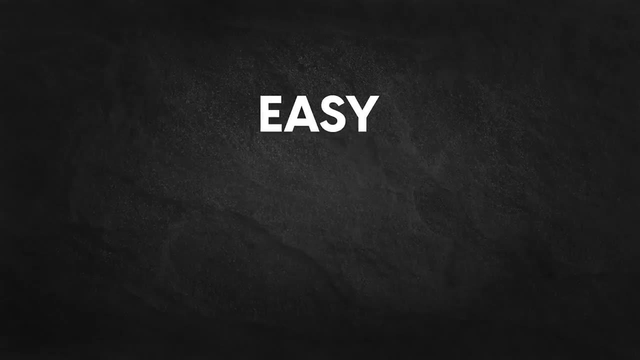 when I encountered my first medium problem. The second and the bigger advantage, according to me, is that when you solve the medium problems, you'll actually learn more from them. Let me explain what I mean by this. Imagine that you have not solved any easy problems and you try to solve a medium. 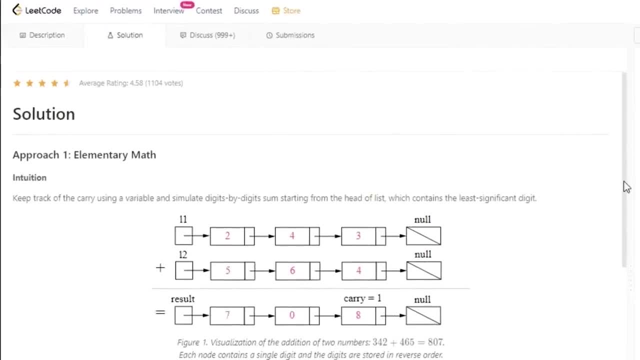 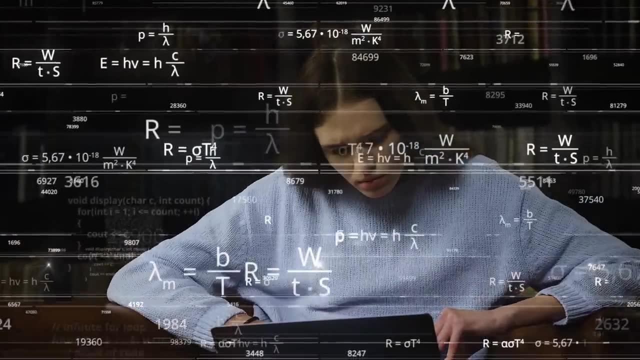 problem. Let's say you are not able to solve the problem and you look at the solution. There's a good chance that you might not be able to understand the solution And you even if you do, it's highly unlikely that you will grasp all the nuances of the solution. So 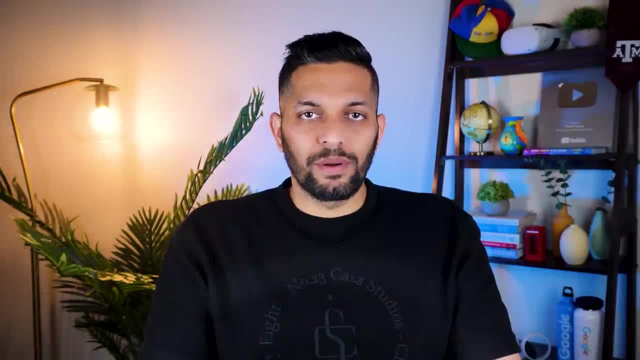 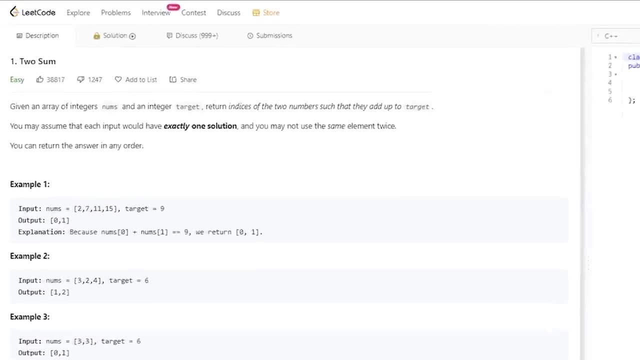 having some easy problems under your belt is a must. before moving to the medium problems, Let's go back to our top interview questions and sort them by difficulty. Solve these 37 easy problems before you move on to the mediums. Now that you know the high level lead code strategy, let's 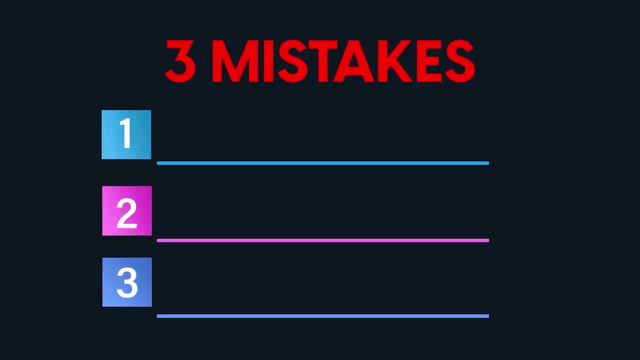 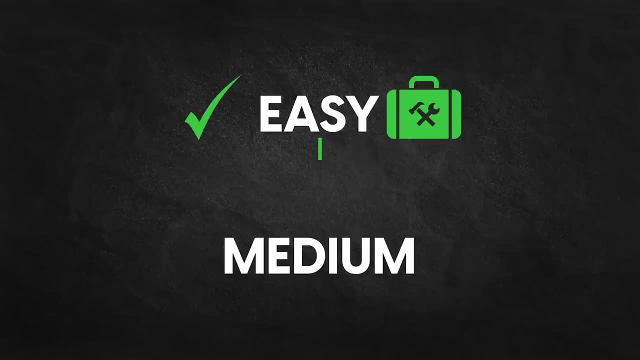 looking to stay motivated and actually improve your programming logic, you have to start with the easy problems. As you solve some easy problems, you'll start collecting some tools for your toolbox And when you reach the medium problems you'll be able to use. 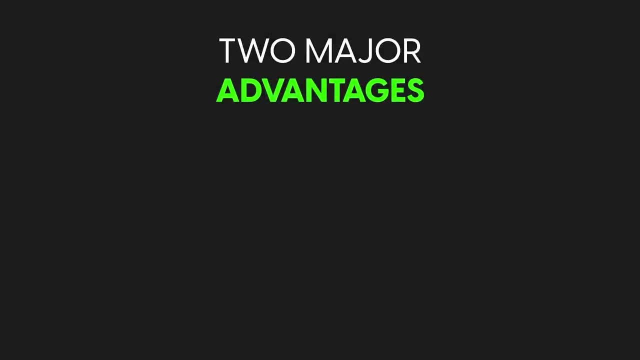 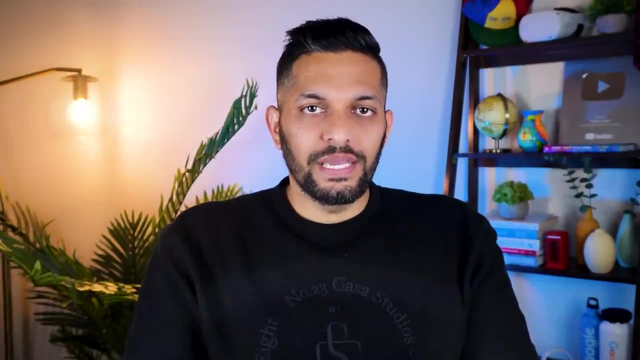 these tools to tackle them. This approach has two major advantages. One: you will not lose your confidence, like I did when I encountered my first medium problem. The second and the bigger advantage, according to me, is that when you solve the medium problems, you'll actually learn more from them. 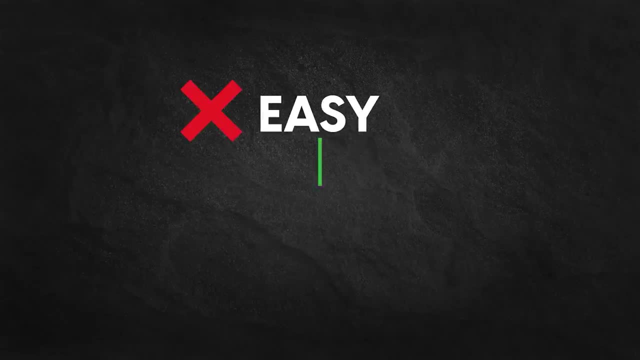 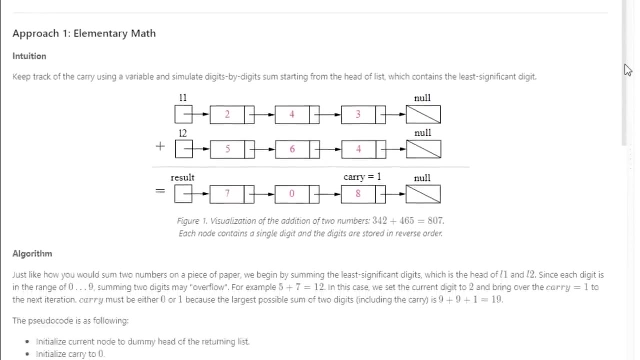 Let me explain what I mean by this. Imagine that you have not solved any easy problems and you try to solve a medium problem. Let's say you are not able to solve the problem and you look at the solution. There's a good chance that you might not be able to understand. 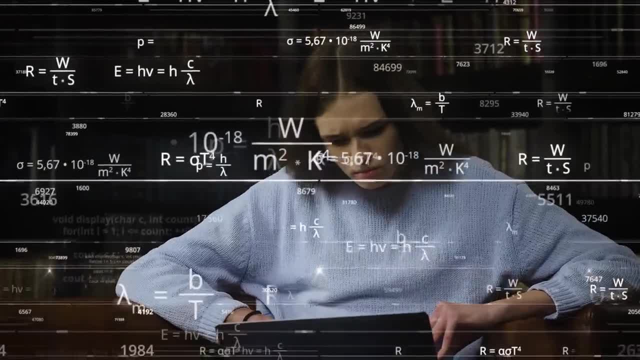 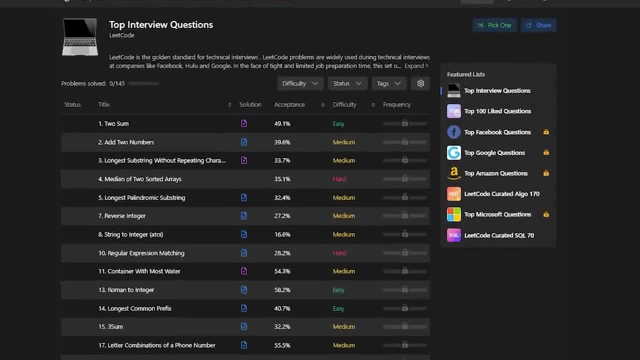 the solution. And even if you do, it's highly unlikely that you'll grasp all the nuances of the solution. So having some easy problems under your belt is a must. before moving to the medium problems, Let's go back to our top interview questions and sort them by difficulty. 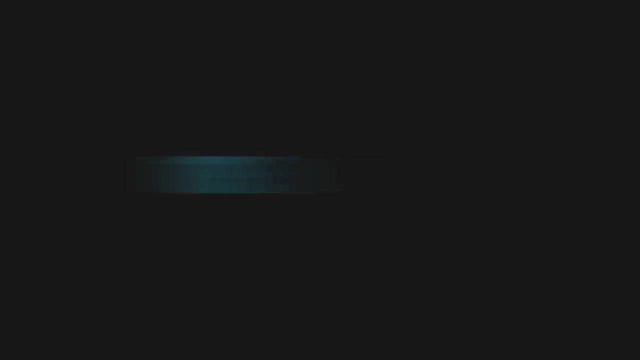 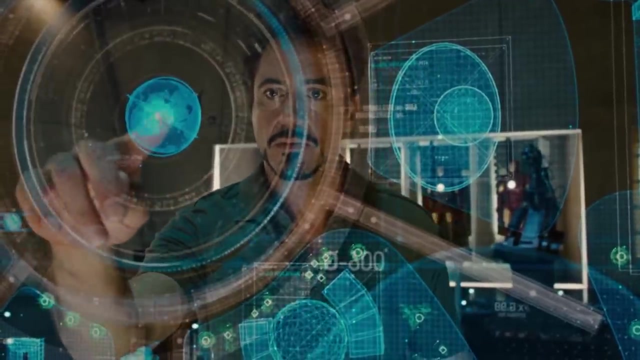 Solve these 37 easy problems before you move on to the mediums. Now that you know the high-level lead code strategy, let's dig a little deeper and see how to approach any new problem. And this is where you see a big difference between a newbie and a pro interviewee. 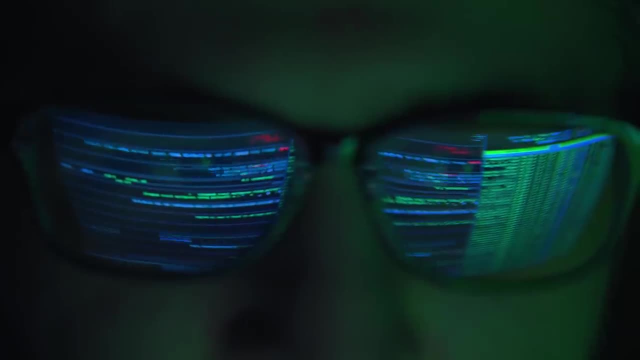 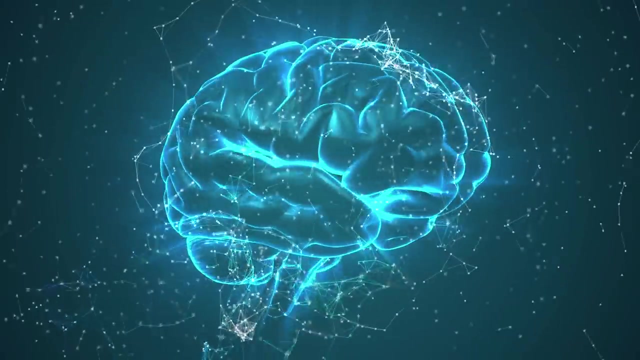 Let me tell you how a beginner solves any new problem. They read the problem statement and immediately start coding a solution. What they don't understand is that we should leave multi-processing to the computers. Our brains are not built to think and code the solution at the same time. 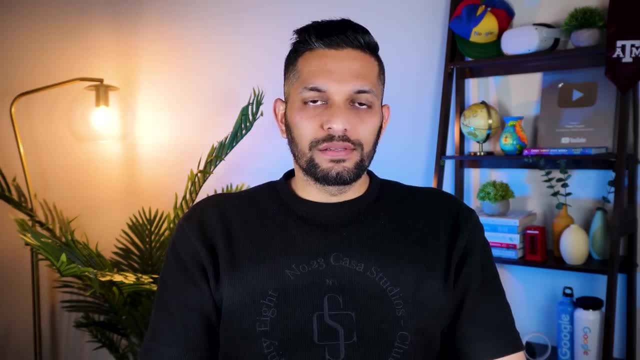 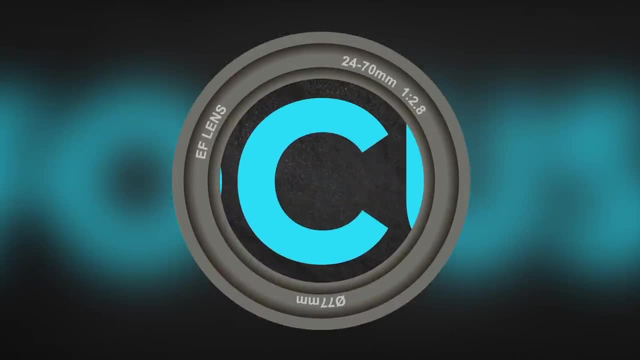 In fact, as much as the productivity gurus would like you not to believe this, we humans cannot multitask. Our focus is like the zoom lens of a camera: We can zoom in to see that one thing, or we can zoom out to see more things, but we cannot do both at the same time. 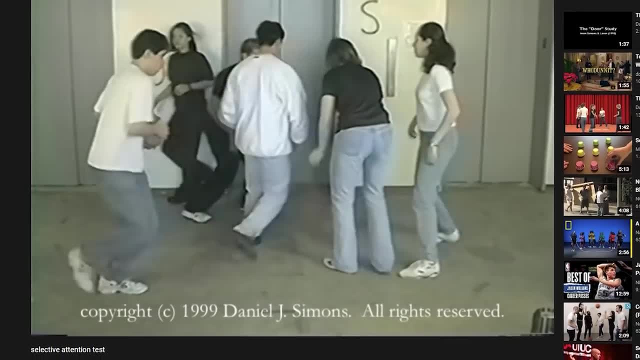 If you don't believe me, you can try out this selective attention test by Professor Simons on YouTube. I will link it in the description. If you are with me on this, I would like you to break the process of solving a coding problem. 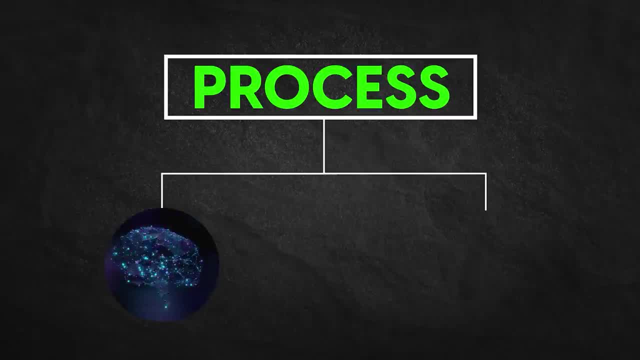 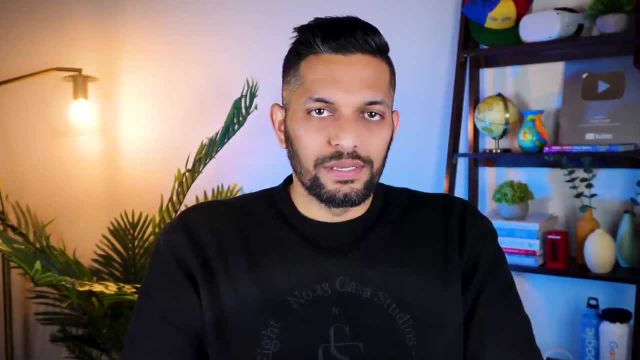 into two separate steps. Step 1 is coming up with the solution in your head, and step 2 is actually coding it up in the editor. Sounds obvious, doesn't it? Well, it's not that simple. You see, when most people are thinking about the solution, what they are actually thinking. 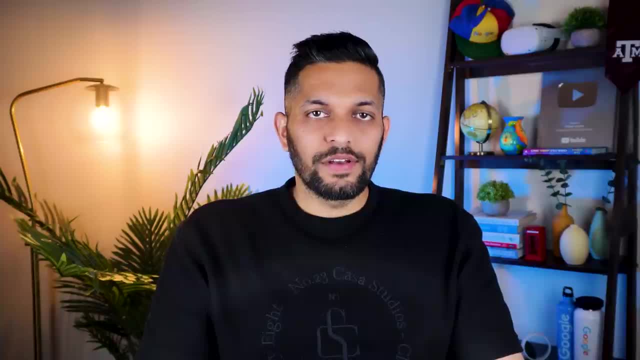 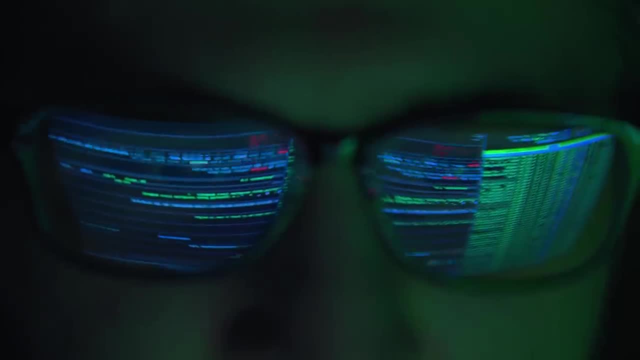 take a little deeper and see how to approach any new problem, And this is where you see a big difference between a newbie and a pro interviewee. Let me tell you how a beginner solves any new problem. They read the problem statement and immediately start coding a solution. What they 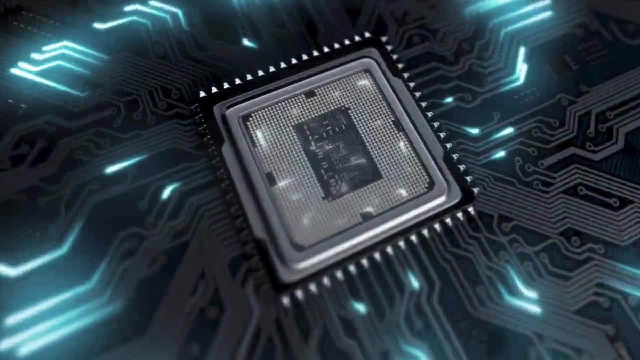 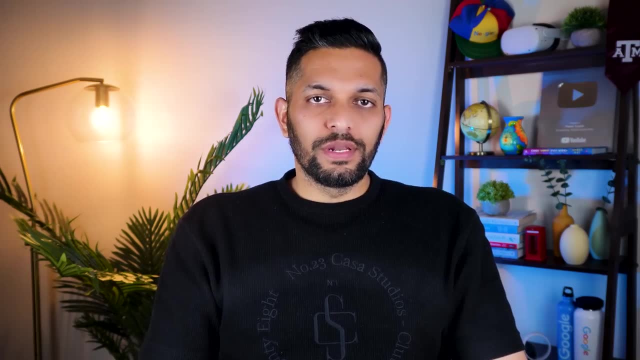 don't understand is that we should leave multiprocessing to the computers. Our brains are not built to think and code the solution at the same time. In fact, as much as the productivity gurus would like you not to believe this, we humans cannot multitask. Our focus is like a zoom. 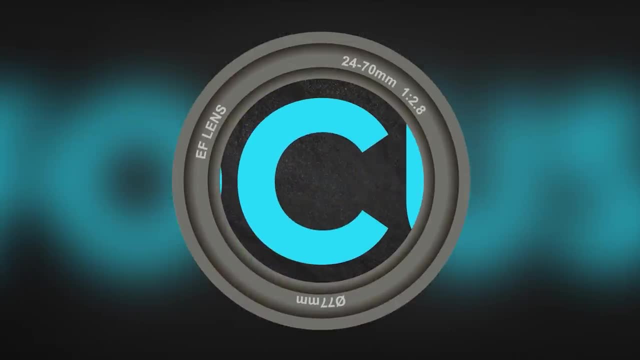 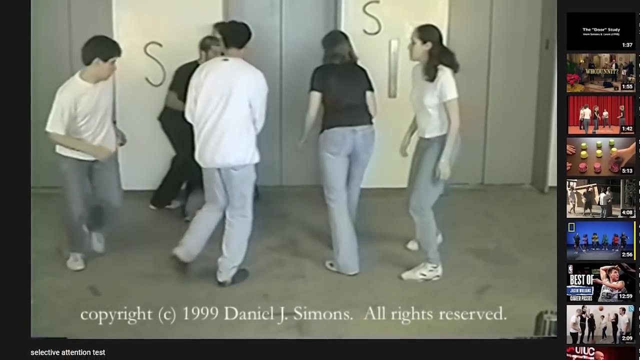 lens of a camera. We can zoom in to see that one thing, or we can zoom out to see more things, but we cannot do both at the same time. If you don't believe me, you can try out this selective attention test by Professor Simon, who is a professor at the University of New York. He 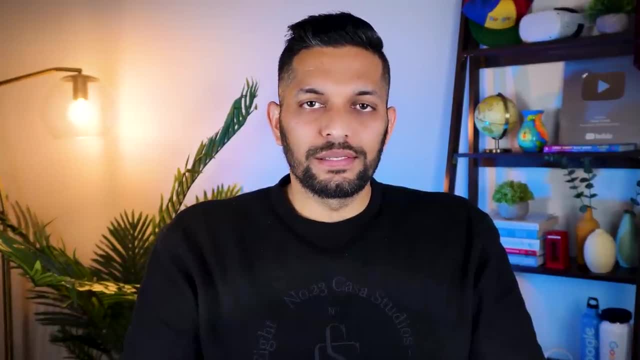 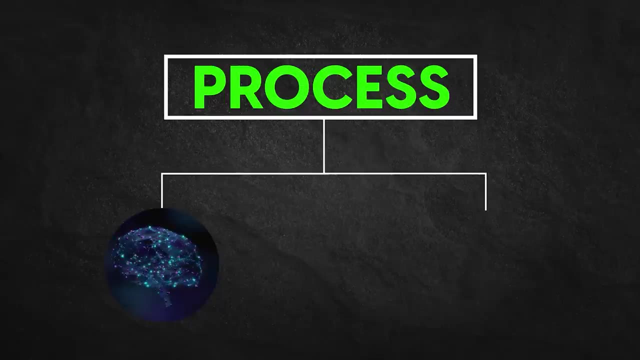 will help you solve the problem. I will link it in the description. If you are with me on this. I would like you to break the process of solving a coding problem into two separate steps. Step 1 is coming up with the solution in your head, and step 2 is 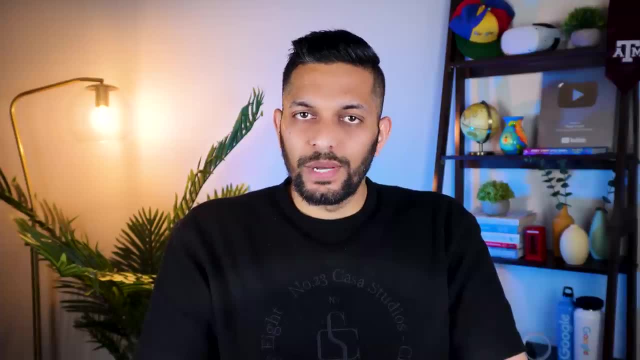 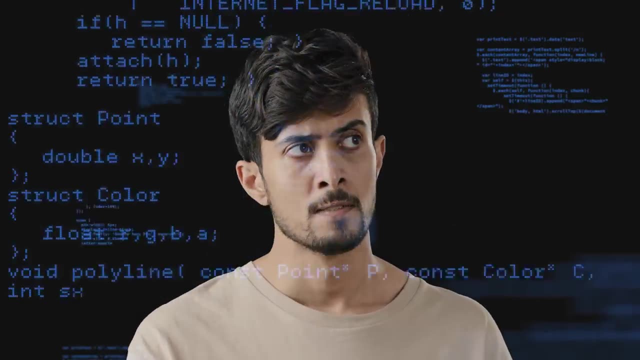 actually coding it up in the editor Sounds obvious, doesn't it? Well, it's not that simple. You see, when most people are thinking about the solution, what they are actually thinking about is how to code their solution, And there is a big difference between the two. To explain what I mean: 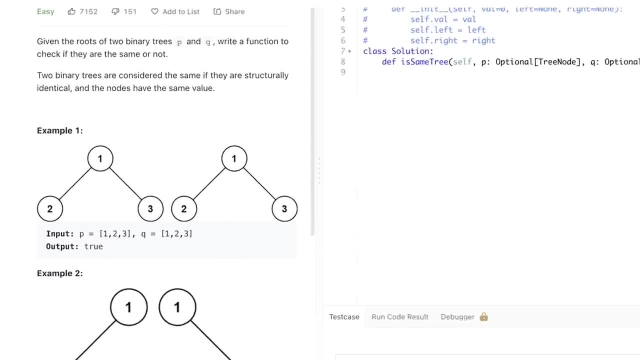 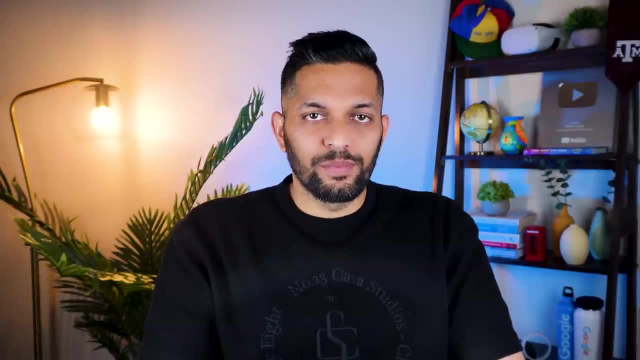 let's walk through this easy problem on lead code. In this problem you are given the root node of two binary trees and you need to tell whether the two binary trees are the same. You can pause the video here if you want to solve the problem yourself. 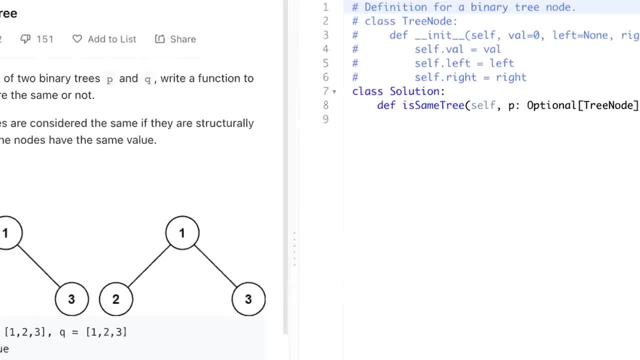 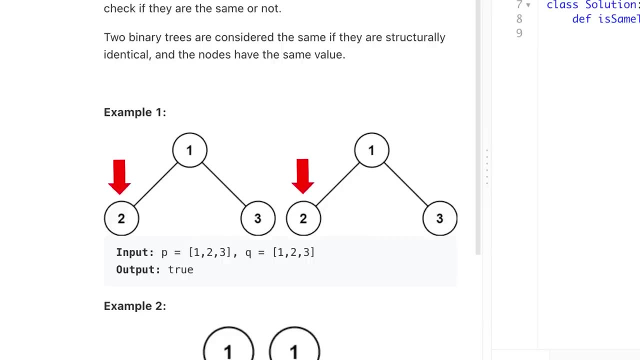 A beginner might look at the given function and start thinking about checking the value at the root node of both trees to see if it's the same. In the next step they would start thinking how they can compare the value of the node to the left or the right of the root nodes. 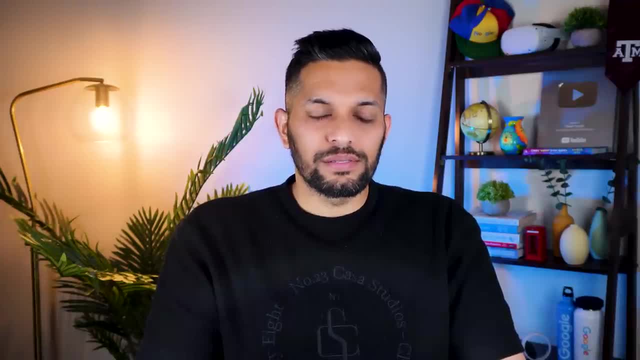 This way of solving might work for this easy problem, but if you are doing this, you are actually thinking about how to code the solution. Now I want you to forget that you know how to code. Think about this: Given the root nodes of two binary trees, what needs to be true for the trees? 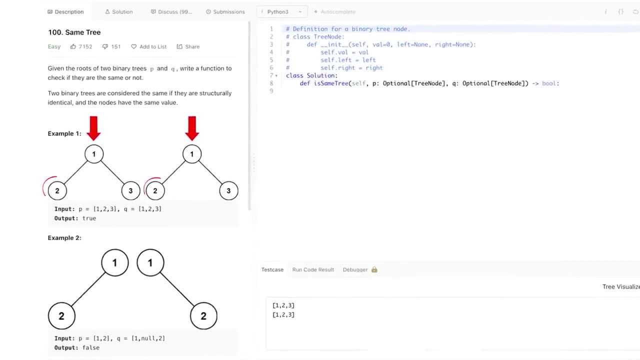 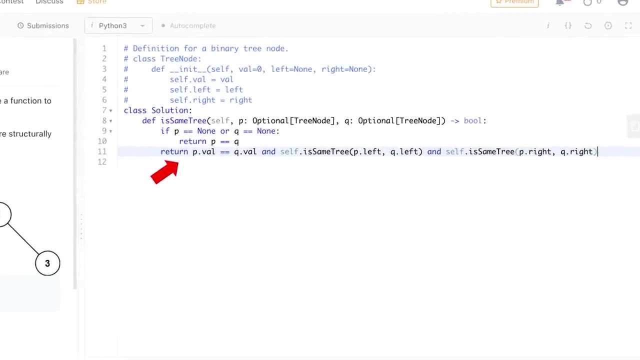 to be same, Value of the root node needs to be the same, the left subtree needs to be the same and the right subtree needs to be the same. Once you see that, the solution is just this one line of code where you check all these three conditions, Training your brain to differentiate. 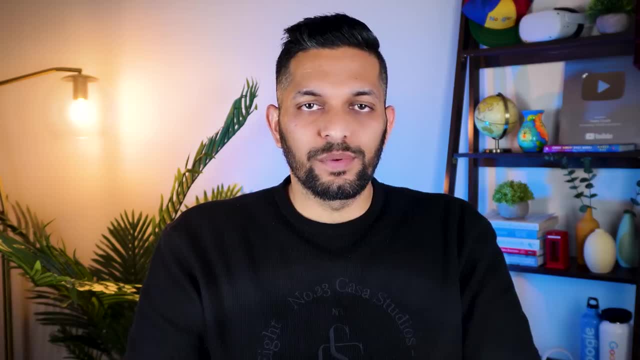 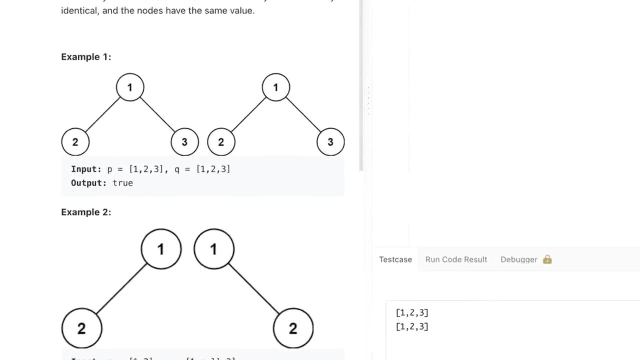 about is how to code their solution, and there is a big difference between the two. To explain what I mean, let's walk through this easy problem on lead code. In this problem there are binary trees and you need to tell whether the two binary trees are the same. 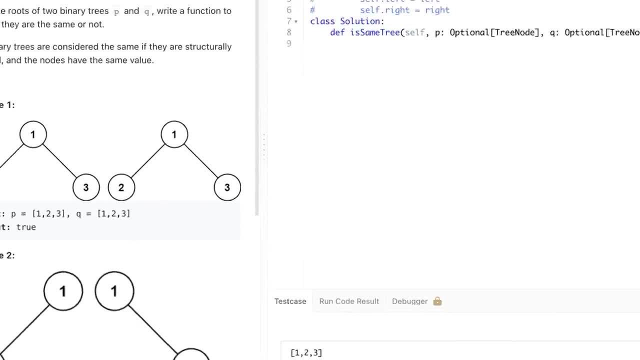 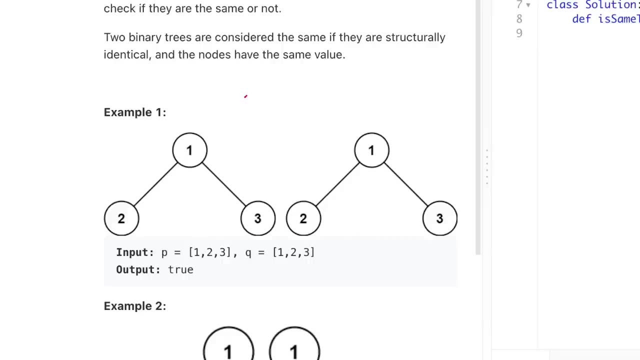 You can pause the video here if you want to solve the problem yourself. A beginner might look at the given function and start thinking about checking the value at the root node of both trees to see if it's the same. In the next step they would start thinking how they can compare the value of the node. 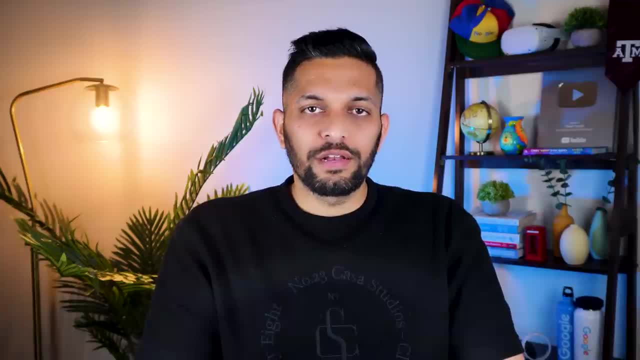 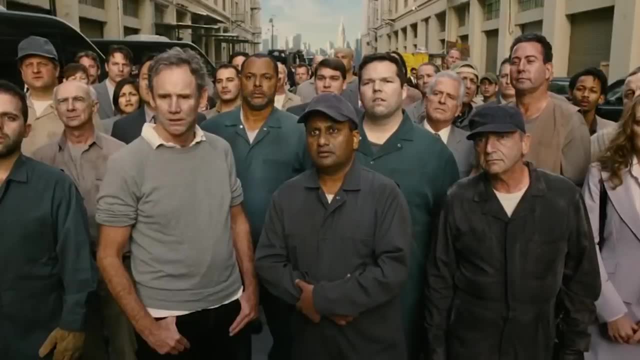 to the left or the right of the root nodes. This way of solving might work for this easy problem, but if you are doing this, you are actually thinking about how to code the solution. Now I want you to forget that you know how to code. 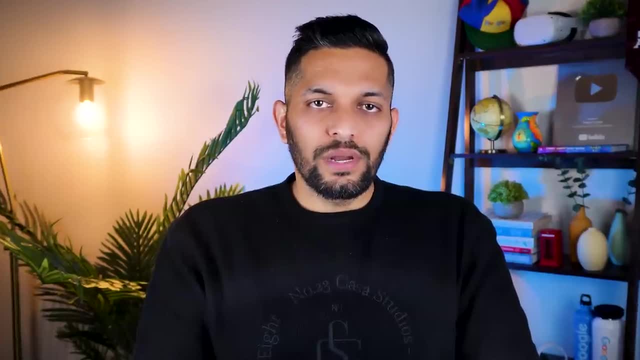 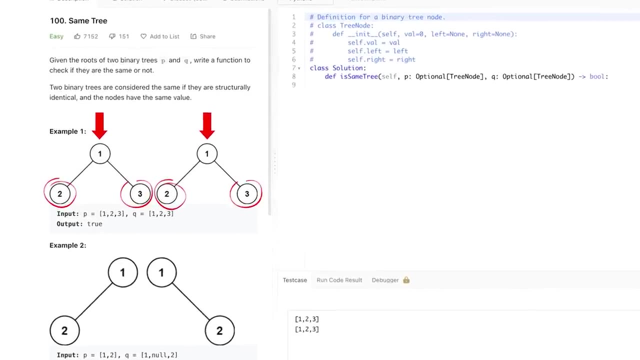 Just think about this: Given the root nodes of two binary trees, what needs to be true for the trees to be same, Value of the root node needs to be the same. the left subtree needs to be the same and the right subtree needs to be the same. 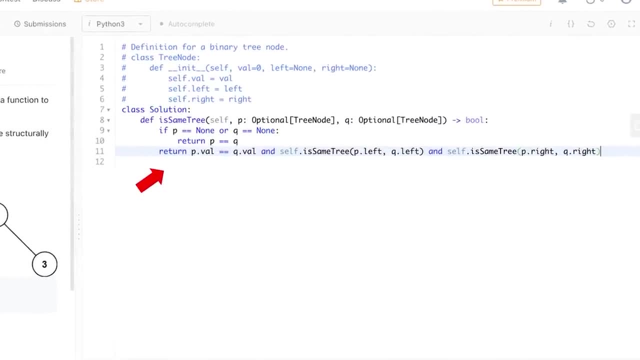 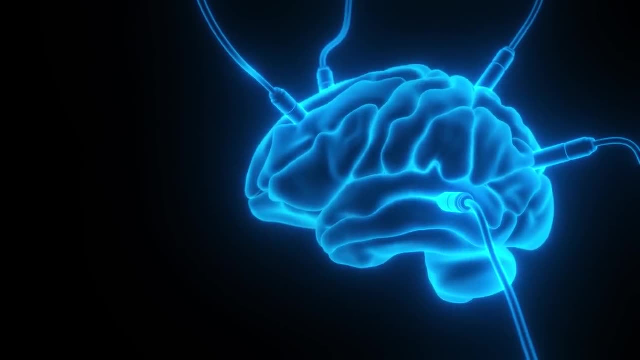 Once you see that the solution is just this one line of code where you check all these three conditions. Training your brain to differentiate between thinking about the solution and coding it up requires a lot of practice, but if you practice enough, you will reach a place where 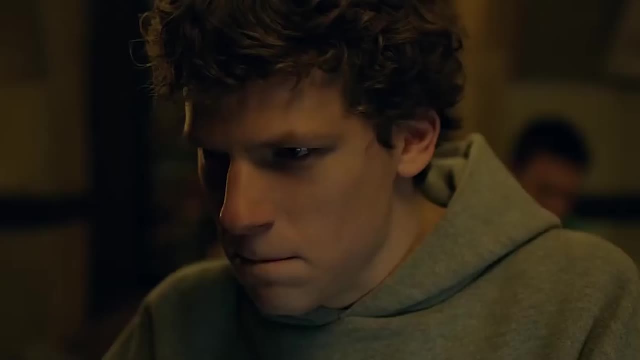 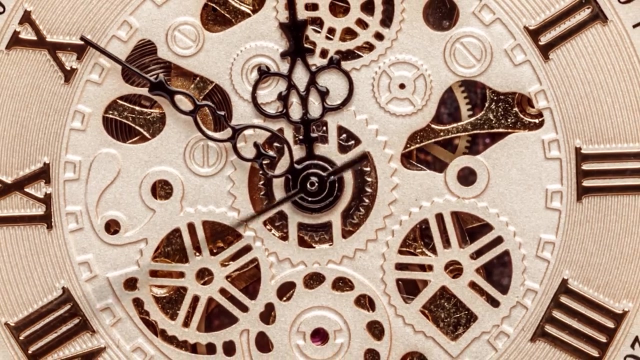 you just have to think about the solution. Once you have a clear solution, the coding part will be done. In my interviews I rarely spend more than 15 minutes writing the actual code. Most of my time goes into thinking about the solution. 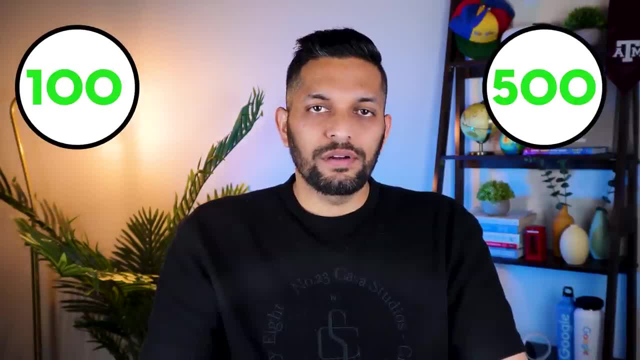 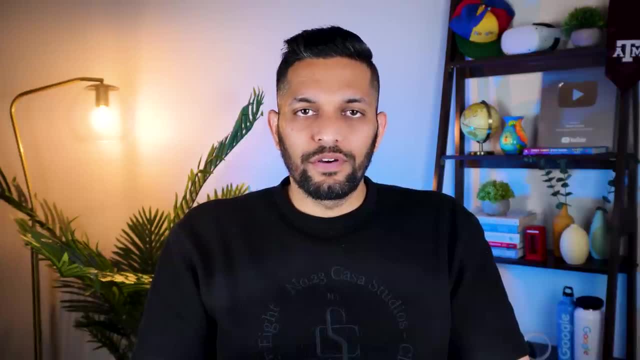 So keep practicing. It might take 100 problems for some and 500 for others, like me, but you will eventually get there. Before we talk about how to know if you are ready for interviews, let's talk about how to actually practice. 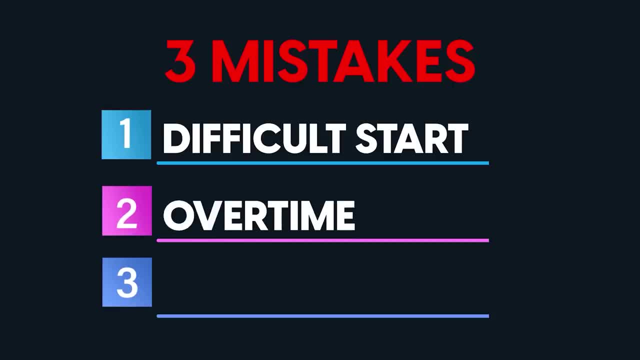 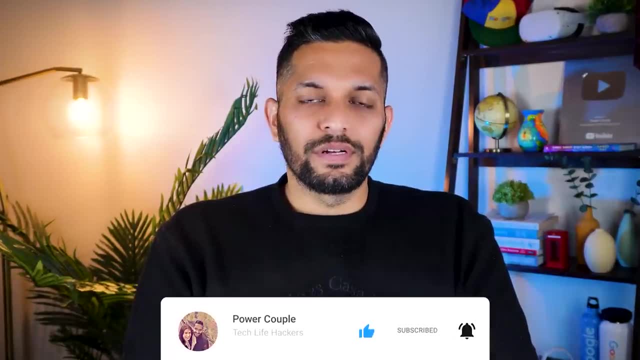 And this is where I made my second big mistake, and that is I spent way too much time on one problem. It was mainly because my ego was very high. How am I not able to solve this easy problem? Maybe if I give it a little more time. 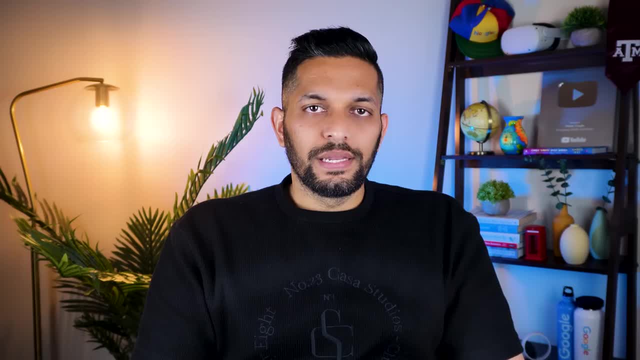 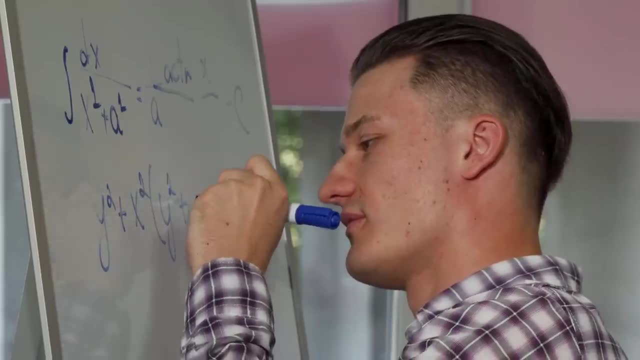 By doing this, I would end up spending up to 3-4 hours on one problem. In an interview, you only get 45 minutes to solve a problem. Why should your practice session be so different? In my opinion, if you are not close to the solution in one hour, you should give up and 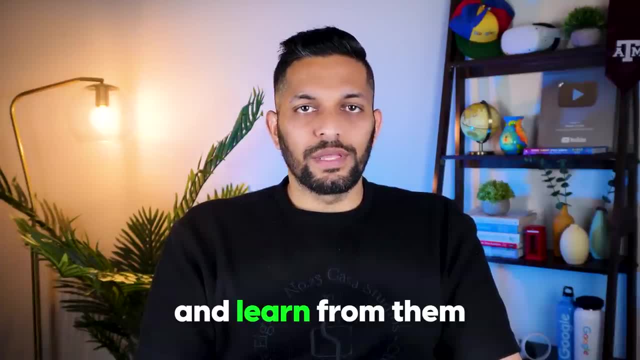 spend rest of the time on looking at the solution of others and learning from them. So go to the discussion section, sort the solutions by most words and read at least top 3 solutions. I recommend 3 solutions and not just the top one. 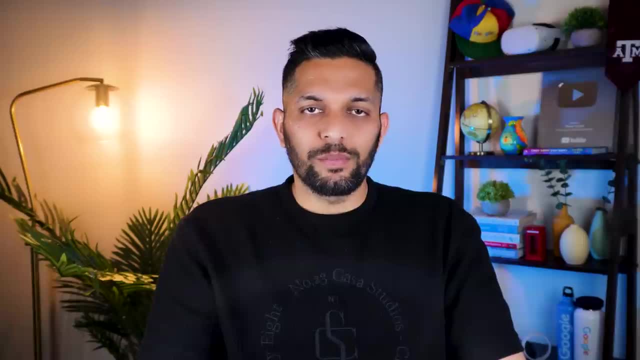 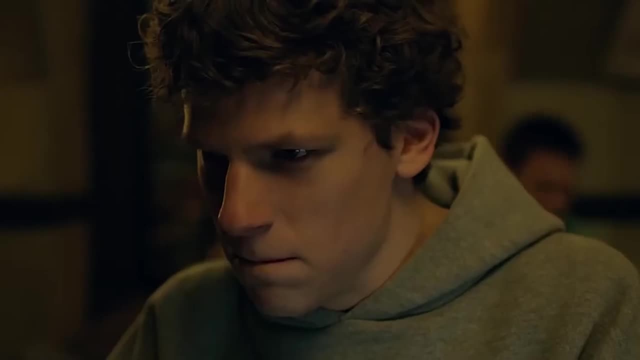 between thinking about the solution and coding it up requires a lot of practice, But if you practice enough, you will reach a place where you just have to think about the solution. Once you have a clear solution, the coding part will start coming naturally to you. In my interviews I rarely 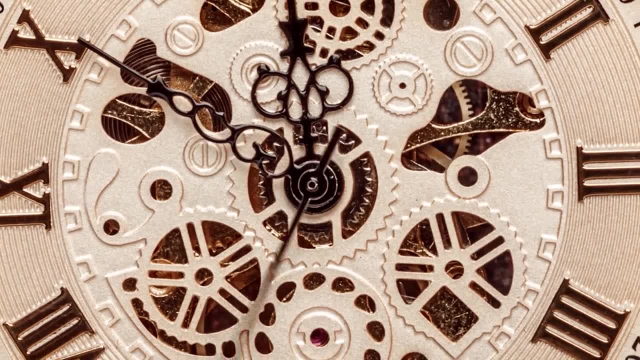 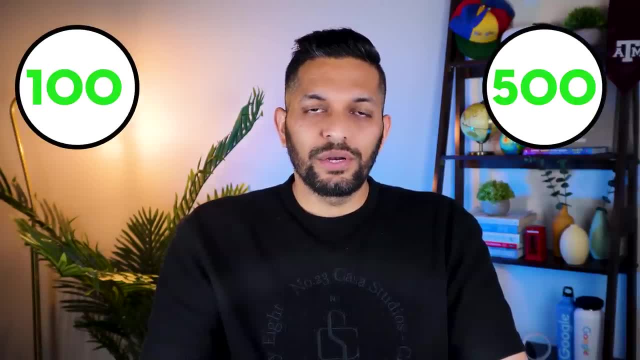 spend more than 15 minutes writing the actual code. Most of my time goes into thinking about the solution, So keep practicing. It might take 100 problems for some and 500 for others, like me, but you'll eventually get there. Before we talk about how to know if you are ready for interviews, 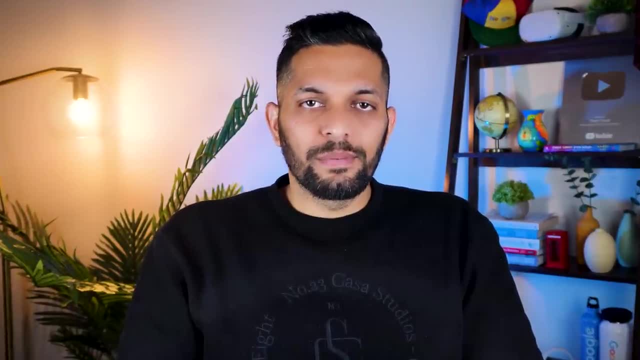 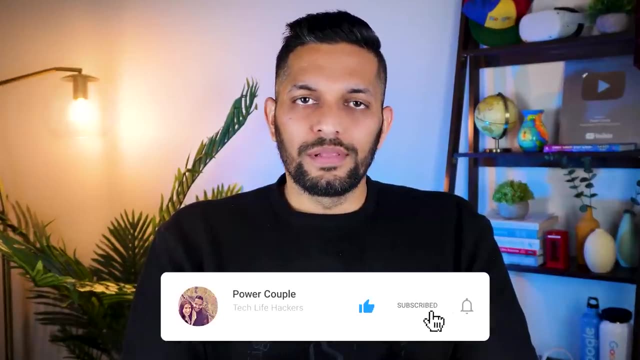 let's talk about how to actually practice, And this is where I made my second big mistake, And that is I spent way too much time on one problem. It was mainly because my ego was very focused on solving the problem. How am I not able to solve this easy problem? Maybe if I give it a. 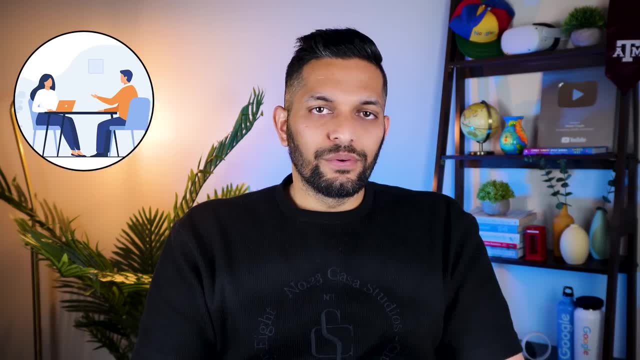 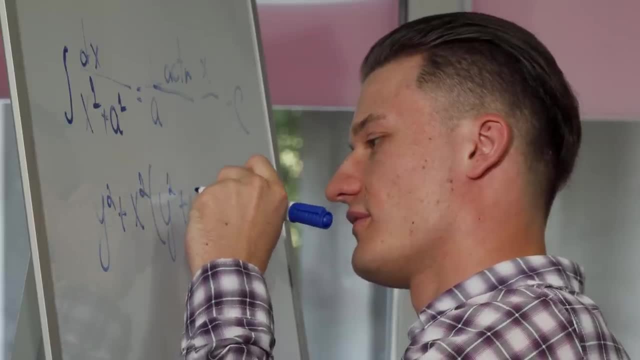 little more time. By doing this, I would end up spending up to 3-4 hours on one problem. In an interview, you only get 45 minutes to solve a problem. Why should your practice session be so different? In my opinion, if you're not close to the solution in one hour, you should give up and 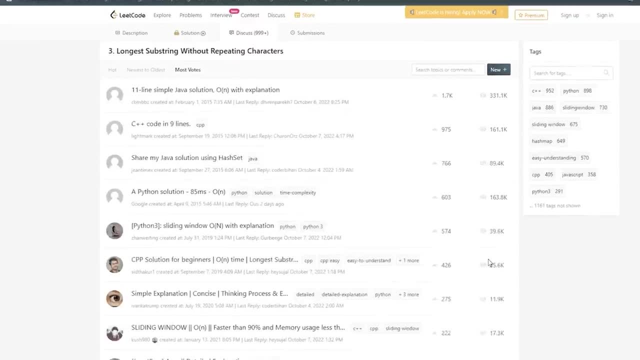 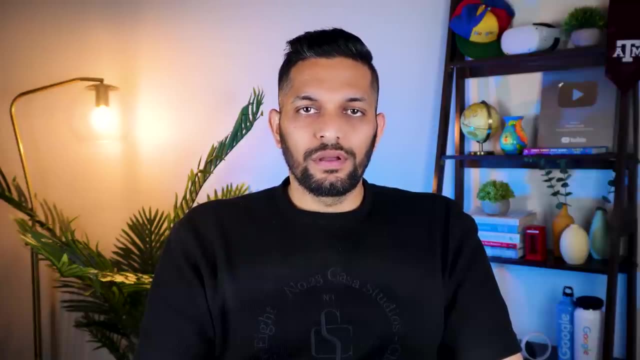 spend the rest of the time on looking at the solution of others and learning from them. So go to the discussion section, sort the solutions by most words and read at least top three solutions, Not just the top one, because sometimes the top solution is not practical for the interviews. 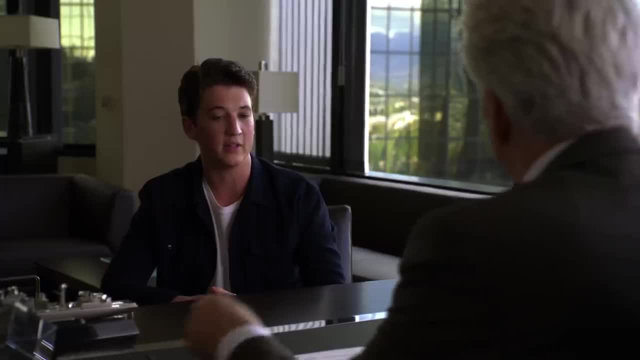 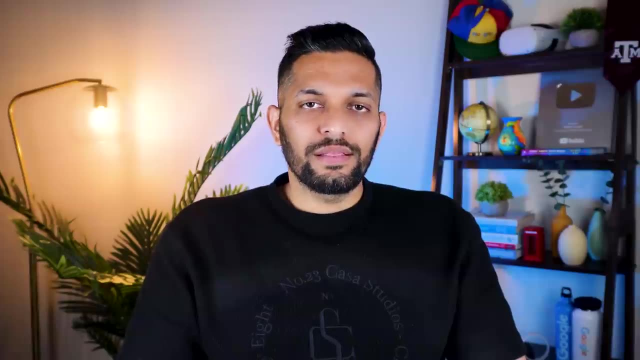 Try to understand the solution rather than memorizing it, because you'll not be able to replicate the solution in the interview. After understanding the solution, come back to the editor and code it up yourself, Even if you think that you're writing the exact same solution that you just read. 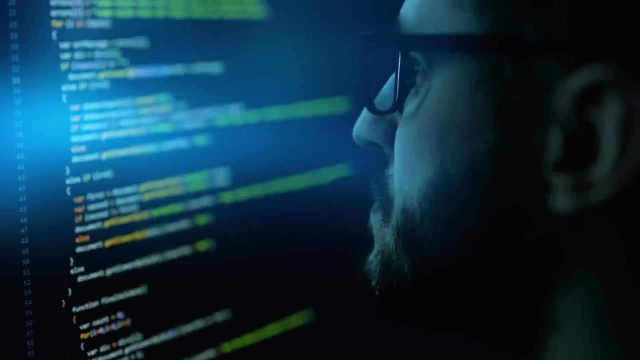 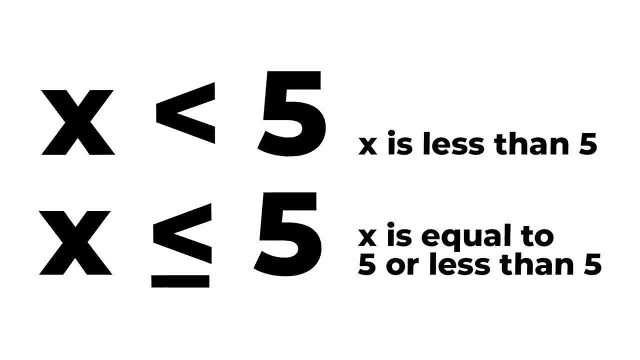 do it. That's because many times there are corner cases that you'll not be able to see by just reading. And when you hit the test cases that don't pass, you will appreciate the difference between less than, less than or equal to much better. 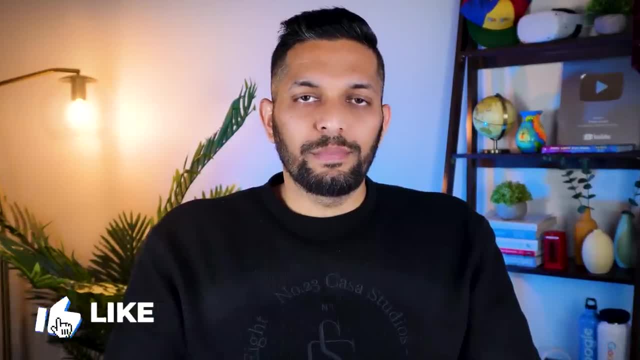 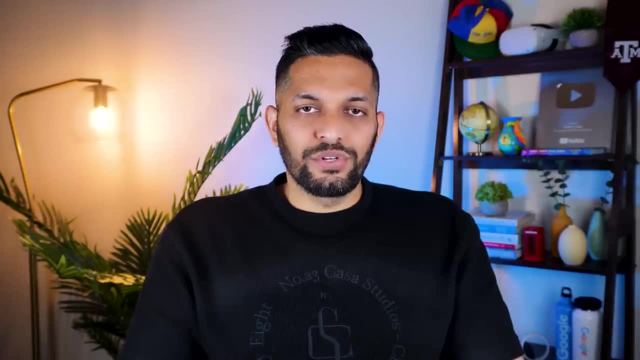 But what do you do if you are able to solve the problem? And this is where I made my third and the final mistake: After solving a problem, I would just move on to the next question. And that is not the best strategy, because your solution might not be optimal. It might pass all the test cases. 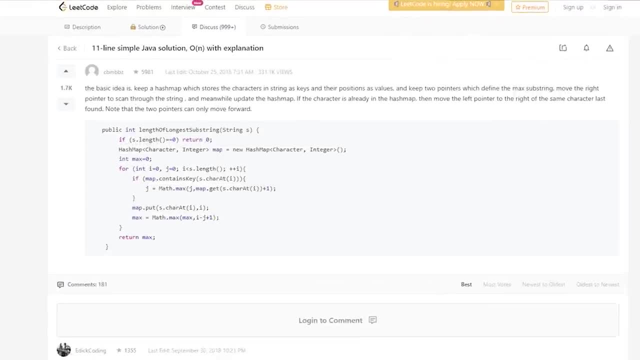 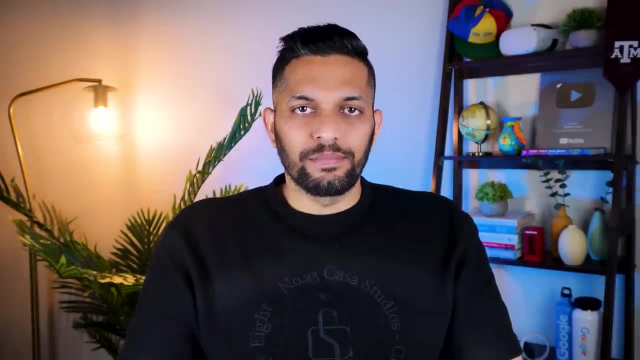 but there still might be some better solutions out there. I recommend reading the top solutions, no matter what. This is especially important if your solution is too lengthy and you think that you cannot solve this problem in the interview time. In my opinion, if you're writing a solution, 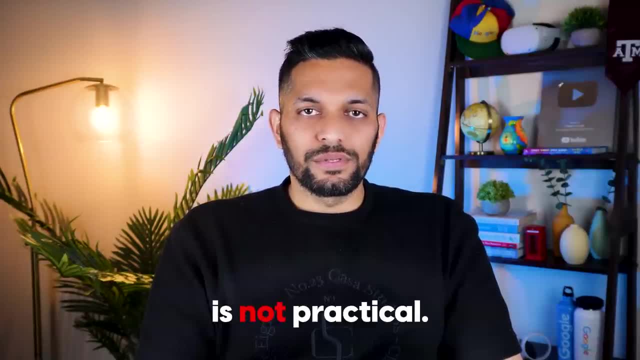 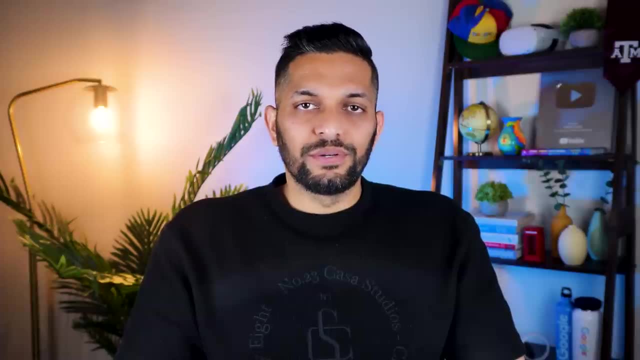 Because sometimes the top solution is not practical for the interviews. Try to understand the solution rather than memorizing it, because you will not be able to replicate the solution in the interview. After understanding the solution, come back to the editor and code it up yourself. 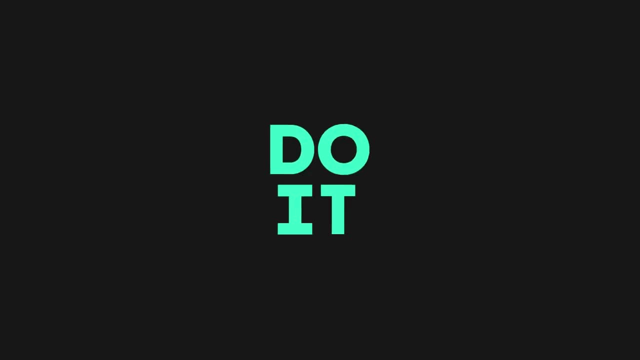 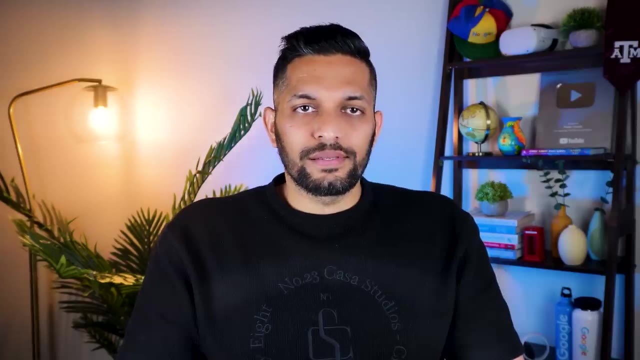 Even if you think that you are writing the exact same solution that you just read, do it. That's because many times there are corner cases that you will not be able to see by just reading, And when you hit the test cases that don't pass, you will appreciate the difference between. 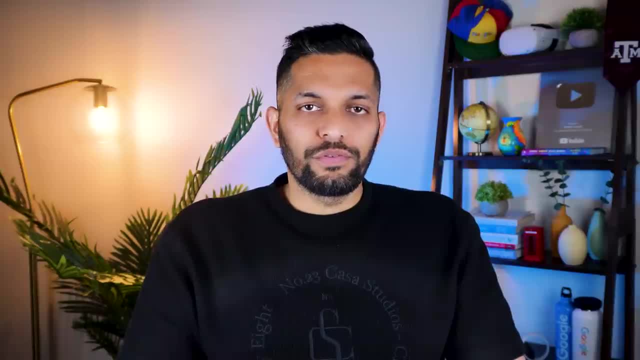 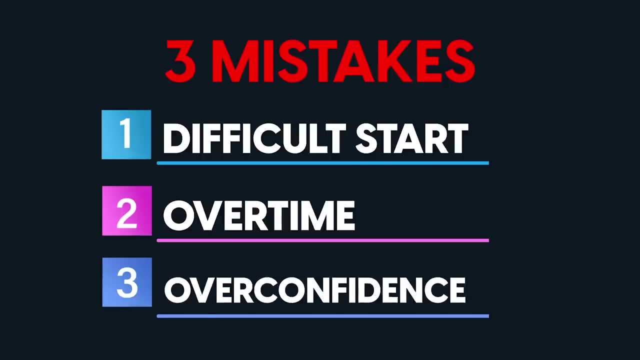 less than, less than or equal to much better. But what do you do if you are able to solve the problem? And this is where I made my third and the final mistake: After solving a problem, I would just move on to the next question. 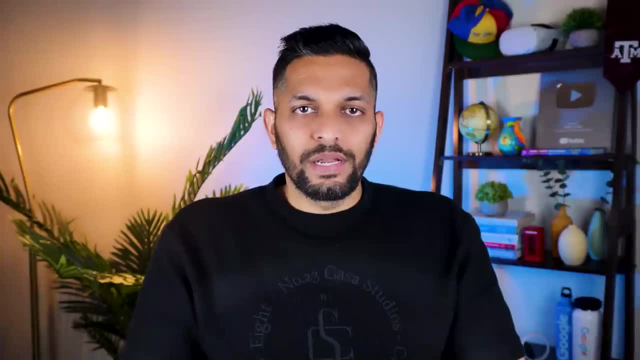 And that is not the best strategy, because your solution might not be optimal. It might pass all the test cases, but there still might be some better solutions out there. I recommend reading the top solutions, no matter what. This is especially important if your solution is too lengthy and you think that you cannot. 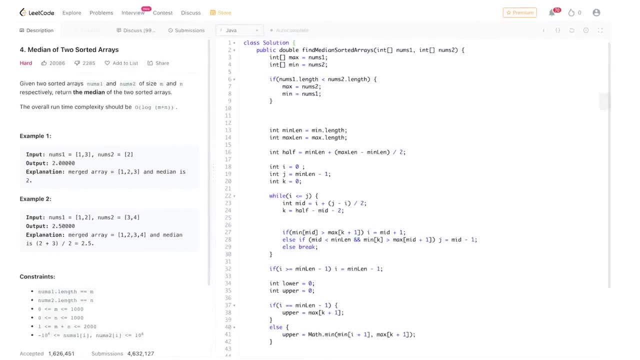 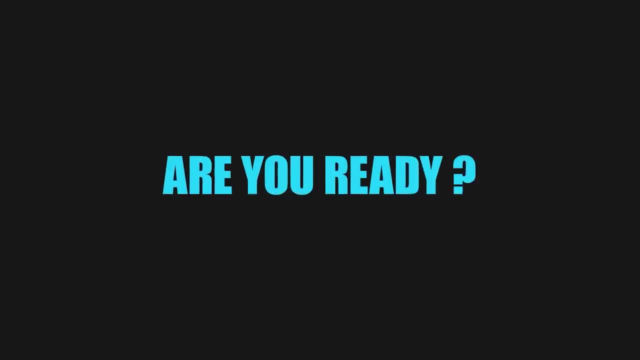 solve this problem in the interview time. In my opinion, if you are writing a solution that is more than 20 lines of code, there is a good chance that there is a better solution out there, So there is no harm in learning from others. 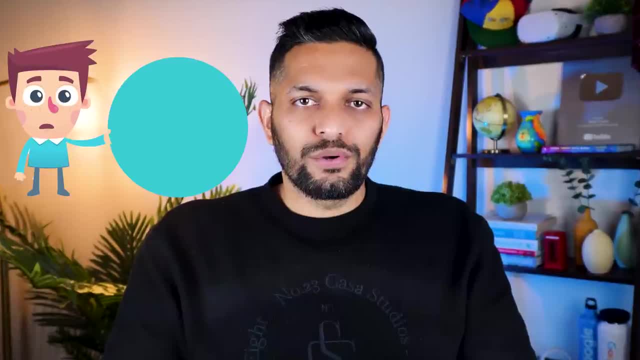 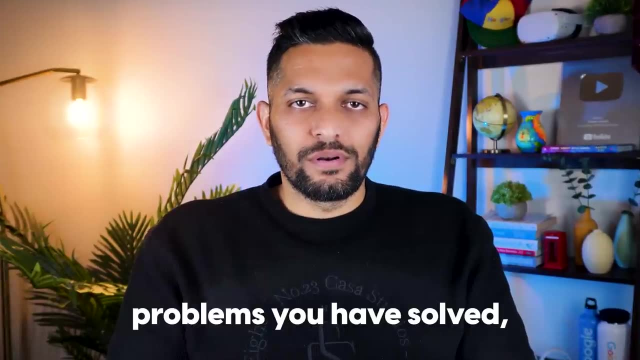 Many people ask me how to decide whether they are ready for coding interviews. Are 200 problems enough, or should I do 500?? To be honest, it doesn't work that way. in life, It's less about how many problems you have solved and more about how good you are at. 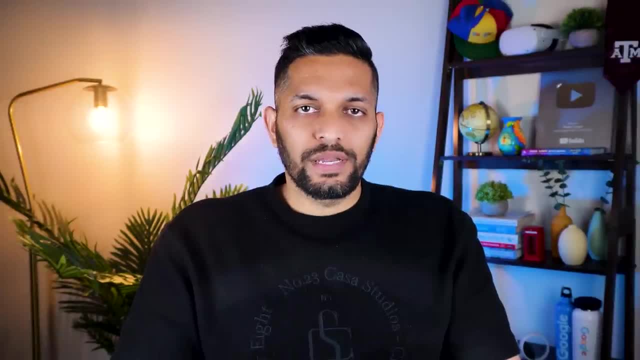 solving any new problem? I believe that we should answer this question from the interview standpoint. An interview is usually 45 minutes long and in most interviews they ask you leetcode medium problems, Accounting for the pressure of the interview and adding a buffer for the introductions. 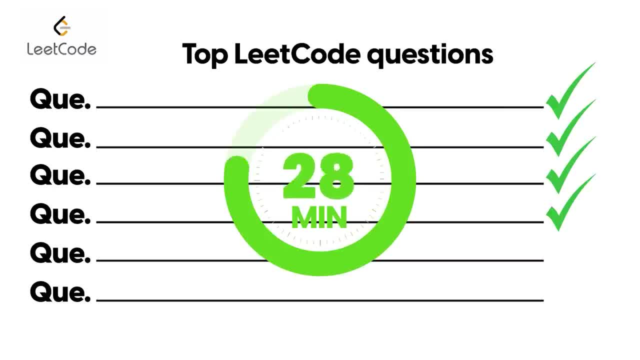 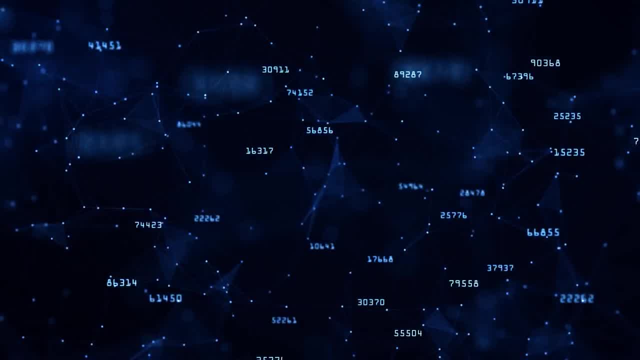 you can consistently solve leetcode mediums in less than 30-35 minutes. You are ready to go. Reaching this level on leetcode is impossible if you don't have a strong foundational knowledge of data structures and algorithms. To learn how I mastered data structures and algorithms, watch this video. My name is Sahil and I will see you in the next one. 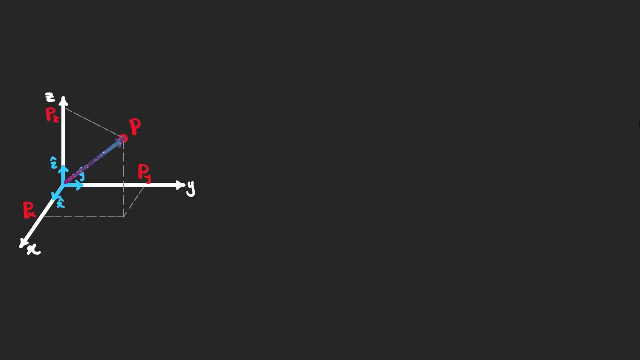 In this video we are going to start with Cartesian coordinate and see what the parameters of a spherical coordinate are. Finally we derive the unit vectors for a spherical coordinate system. Suppose that we have a point in the space. We can define three perpendicular axes- x, y and z. to